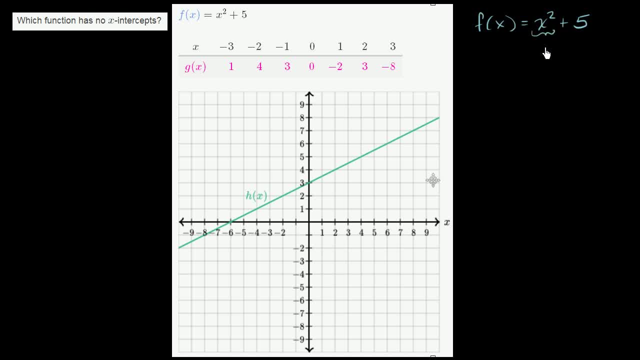 So this is interesting: x squared is always going to be a non-negative number. It'll be 0 or greater. Even if x is a negative value, this is going to be 0.. 0 or greater, And 5 is obviously positive. 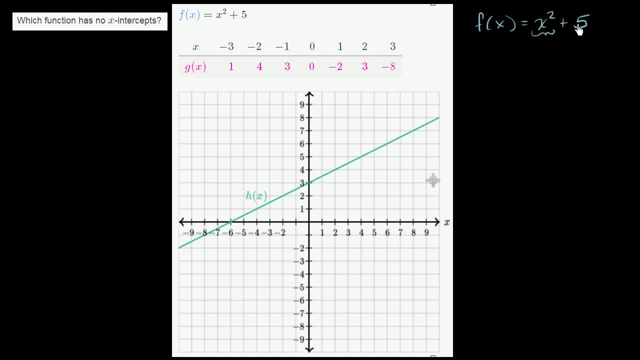 So this whole value or this whole expression, x squared plus 5, is always going to be greater than or equal to 5.. So we could say f of x is always going to be greater than or equal to 5.. So f of x is never going to be equal to 0.. 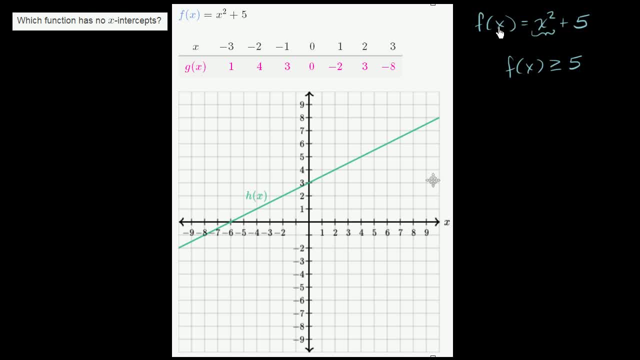 If you don't believe me, let's try it out another way. Let's set f of x equals 0 and figure out which x that might be true. So we could say: 0 is equal to x squared plus 5.. We could subtract 5 from both sides. 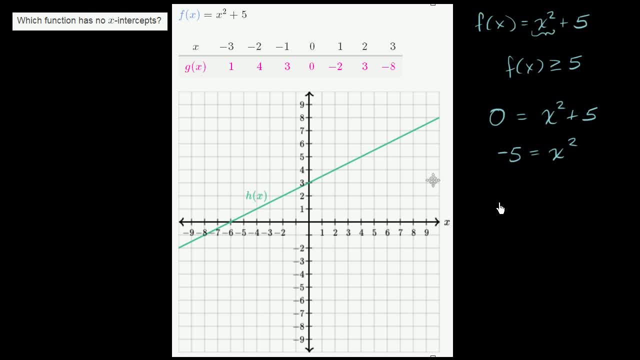 You would get: negative 5 is equal to x squared And if you take the principal root of both sides you've got the principal root of negative. 5 is equal to x. You could even have the positive and negative principal root of negative 5.. 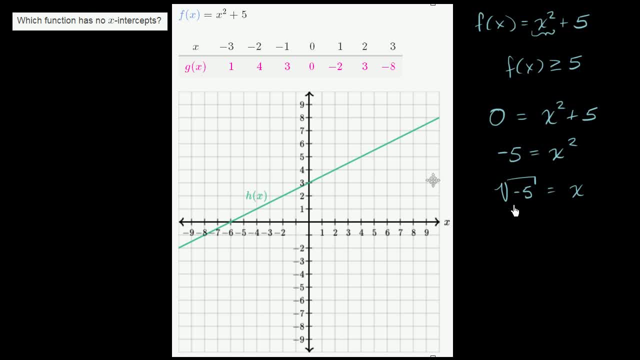 But needless to say, if you're dealing just with real numbers, there is no real number that is the square root of negative 5. So f of x has no x-intercepts. So this right over here it meets the criterion. This right over here has no x-intercepts. 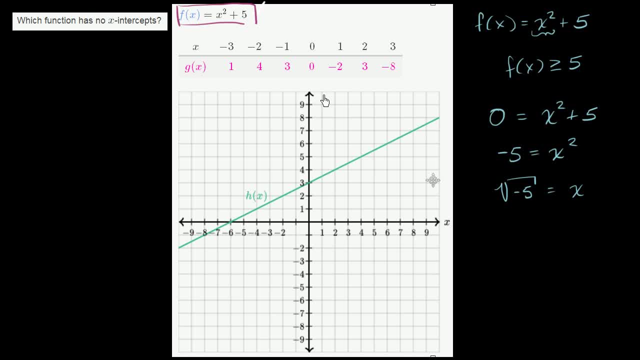 Let's see if these other ones have x-intercepts. So remember, you have an x-intercept if the value of the function is 0 at some point. And we see right over here this function g of x is really defined with this table. 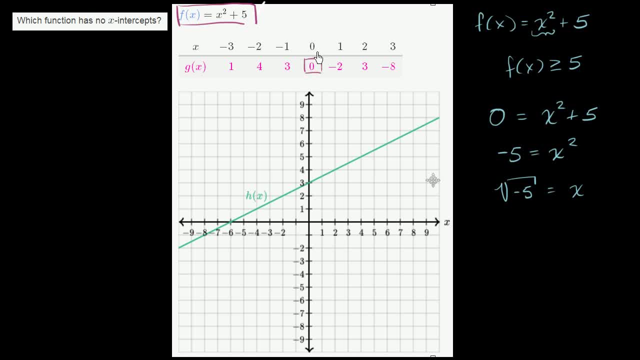 And we see it does indeed equal 0. It happens to equal 0 when x equals 0. So it intersects the x-axis right over there. That's its x-intercept. Now let's look at this green function: h of x. 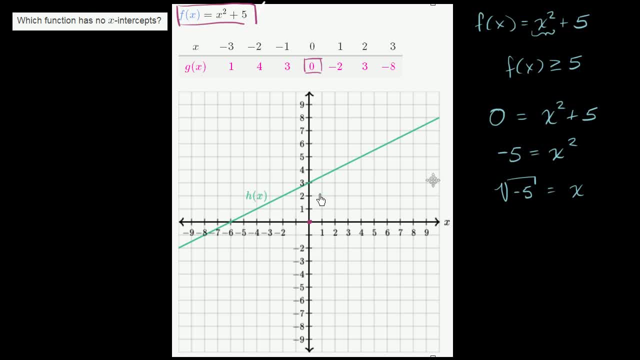 Where does that intersect the x-axis? Well, that's visually more obvious. It intersects the x-axis right over here. h of x is 0 when x is equal to negative 6. So these last two functions have x-intercepts. This first one does not.